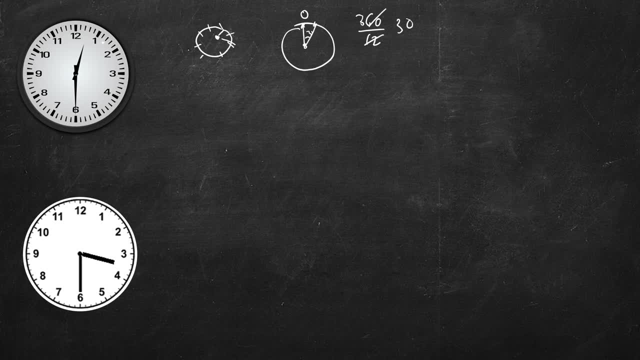 That is 30. So this angle is 30 degree. Similarly, if we reach from 1 to 2, we traverse another 30 degree. That is total 60. And when we reach 3, we traverse another 30 degree. 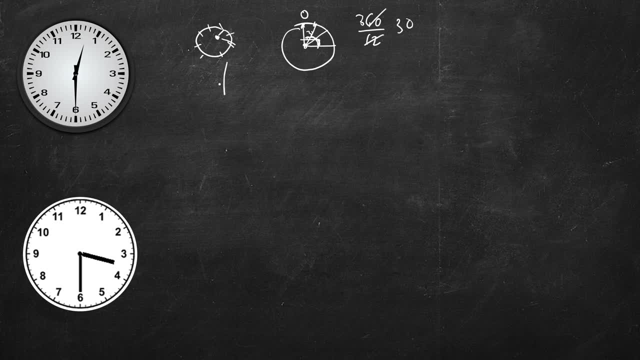 That is total 90.. And you can see that this is 90 degree. 90 degree means perpendicular, So this will be used for our calculation. So this is 30 degree per hour And this need not be integer. If this is one, if this is 0.5 hour, then it will be 15 degrees. 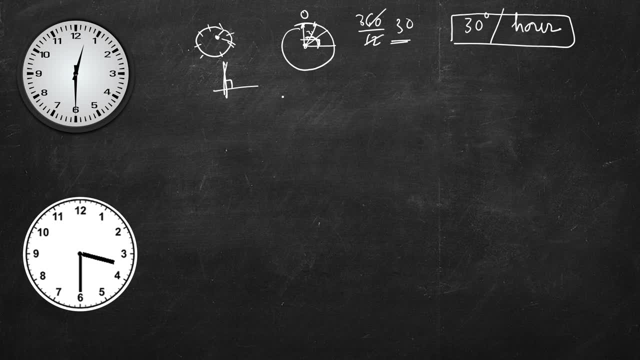 So you can adjust this. So, per hour, 30 degree. Next, what is the angle subtended by per minute? Uh, so again, we have 60 minutes in This entire circle. So here it's 0 minute, 1 minute, 2 minute, here it's 30 minute. 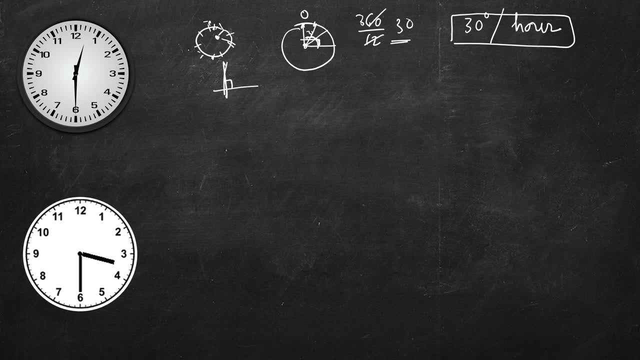 And finally- uh, till here just before this- it's 59 minutes. And when it reaches this 60 minute we increment the hour and make minute to 0.. So 360 degrees divided into 60 minutes, So it's 6 degree. 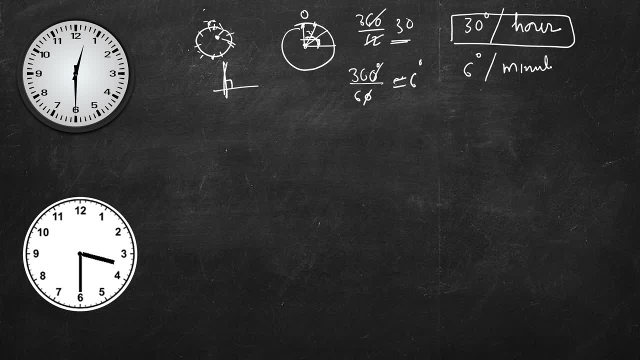 So 6 degrees per minute. In fact, we will not be considering this also. Uh, we will just consider: uh, what is the hour and what is the minute, and our, we will calculate it as our equal to given our- and I forgot to tell the input. you will be given one hour variable and one minute variable, and both will be integer. 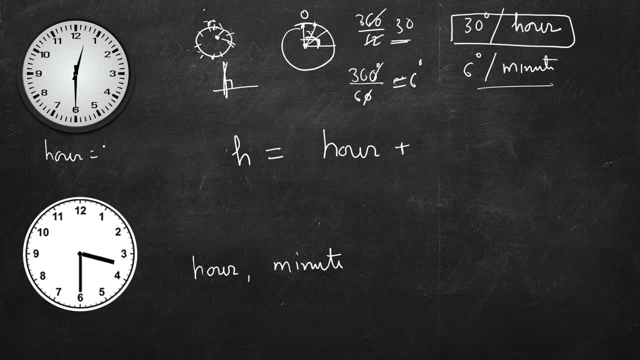 So in this case the input will be our equal to 12, minute equal to 30.. This is the time, And here our is our three, And minute is again 30. So these two integers will be given. So when, uh, the minute is not zero, if minute is zero, the hour handle will be exactly on one of these numbers. 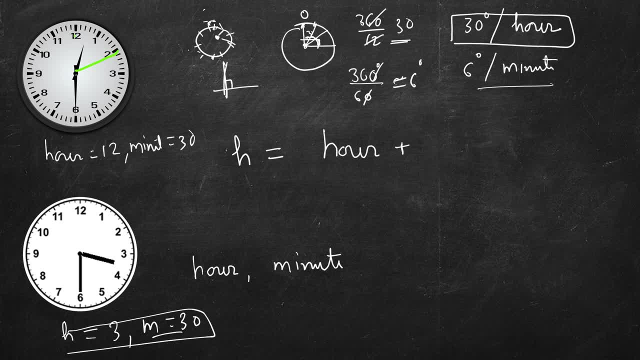 But if minute is not zero, then it will increase to the next value of our, appropriately. What is the minute? in this case? It's 30. So it's exactly half hour. So it's exactly between 12 and one. So what is total hour? 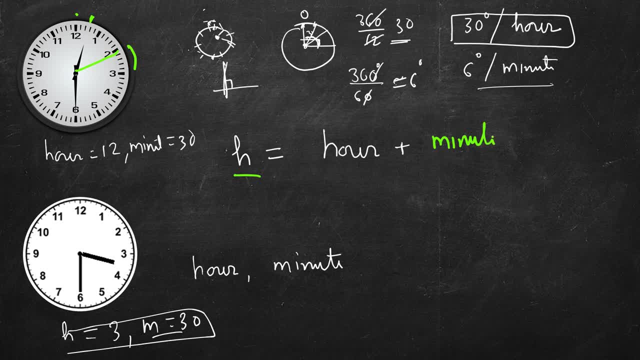 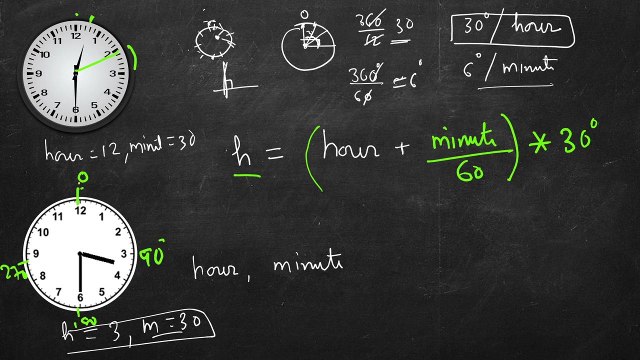 Hour Hour is hour plus minute divided by 60. So this is the total hour And if we multiply it by 30, we get: uh, where is this hour hand? So we will start from: this is zero, this is 90, this is 180 degree, 270 degree and this is 360 or zero. 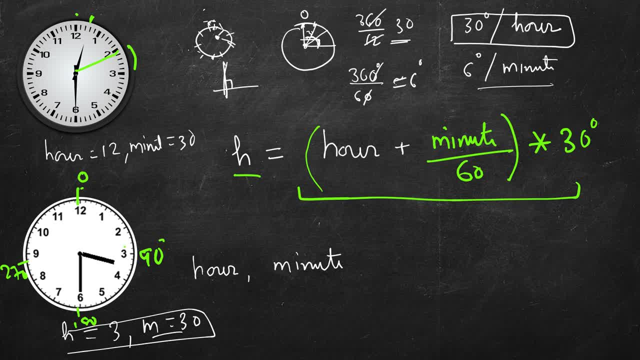 So we will find what is the position. Okay, So this is the position of hour handle. Next, we will find the angle subtended by minute handle. So this will be simply minutes multiplied by six, Since each minute angle between each minute, this is small, two divisions. 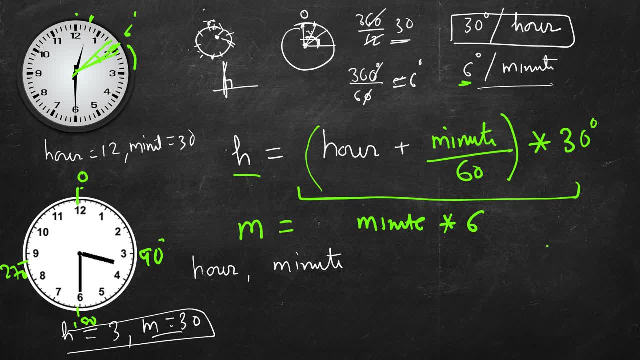 If you see this, this angle will be six degree, So minute multiplied by six. So this is the position of minute handle. So you take the difference, So angle equal to h minus m. Okay, Okay, You take the absolute value of this. 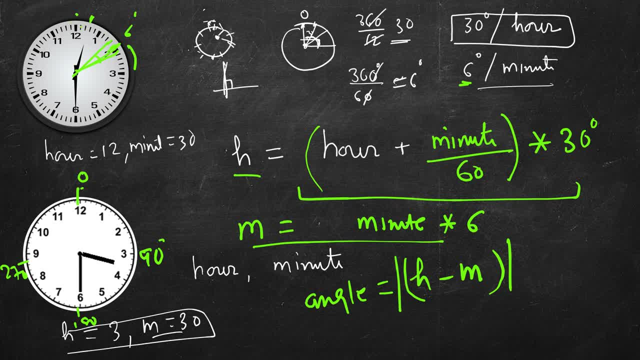 So what is the maximum It can be? it can be here, just before this: three, 60, let's say three, 59 degree, and this can be the minimum, let's say one degree. So what will be the difference here? Difference will be three, 58 degrees. 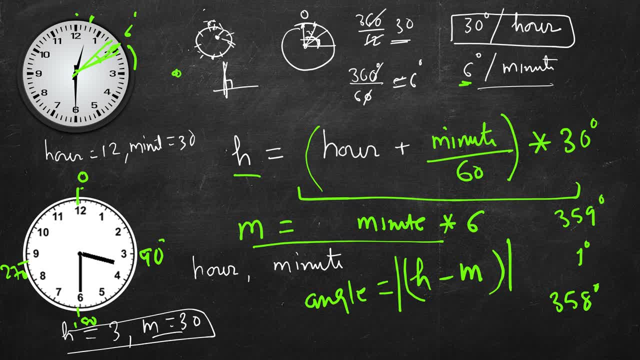 And we need to know that this is more than one 80.. So if our calculation is like this, there are two angles, always one bigger, One is smaller. One will be more than one 80.. One will be less than one: 80.. 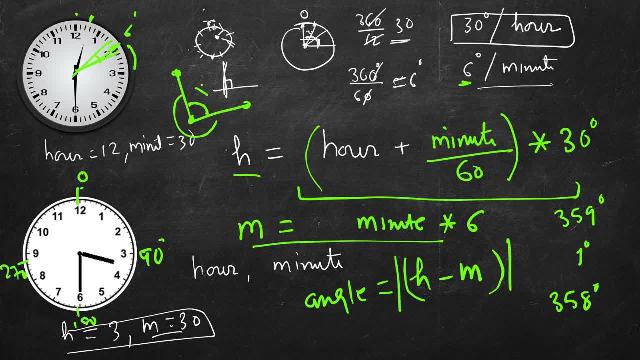 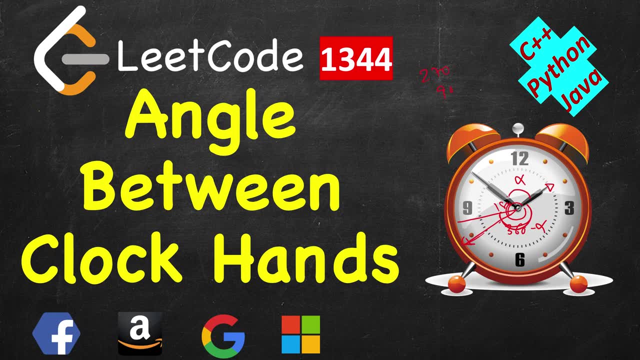 If they're exactly equal, both will be one, 80. So we have to return this one, the smaller one. So if it's more than one 80, what we do? this angle is alpha. This angle is three, 60 minus alpha. 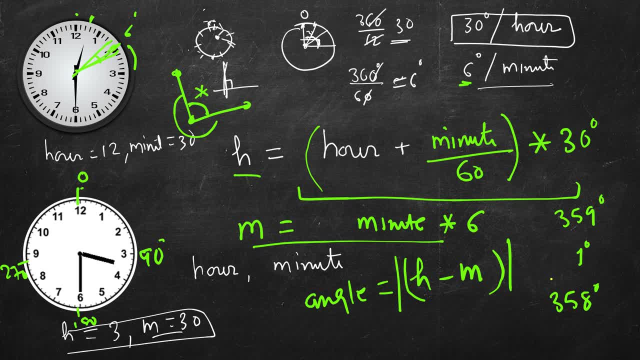 So instead of this angle, we will return three 60 minus this. So subtract it from three: 60. So we will get two degrees, and that is indeed the smallest angle. The minute was here at one minute, or not Even at one minute. 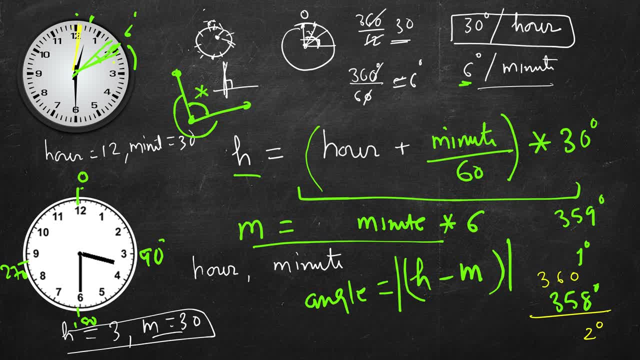 Yeah, It was here at one degree and these minutes are in, uh, integer, So it cannot be in this one degree. It will be at least six degree. So minute was here at six degree and hour was somewhere here. So you can see, indeed, this is a small angle. 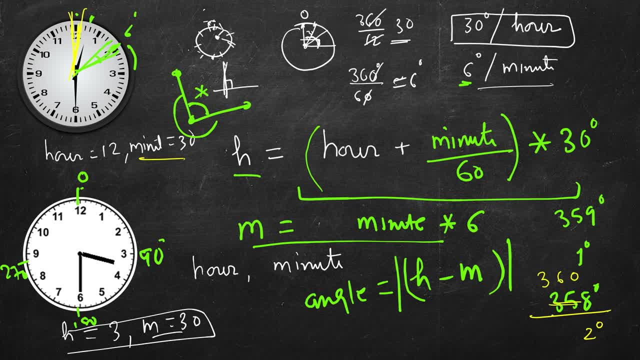 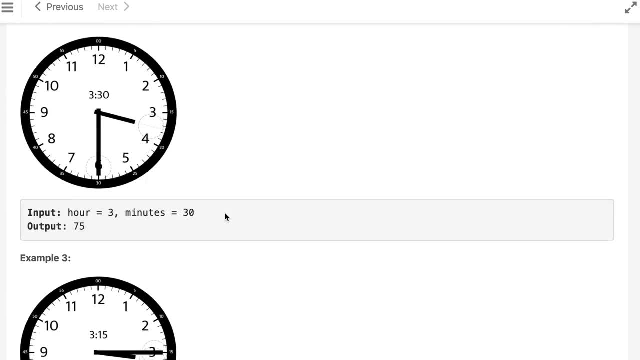 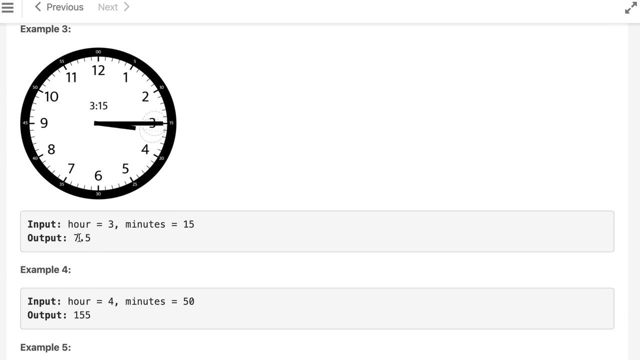 So this three 58 cannot be possible. but you can get the idea. if it's more than one, 80 subtract from three, 60, and that's it. there is no more trick here. So let's write the code for this quickly. So these are in integers, but from here you can see that, uh, the output can be in decimal. 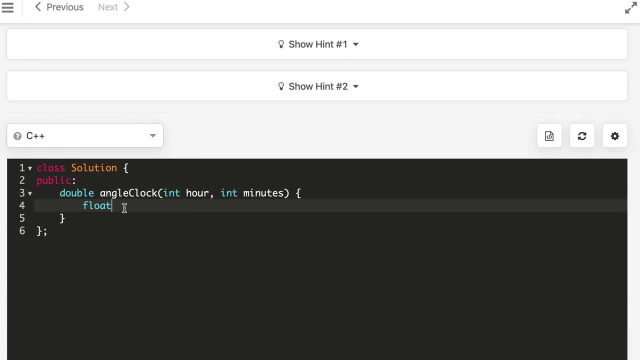 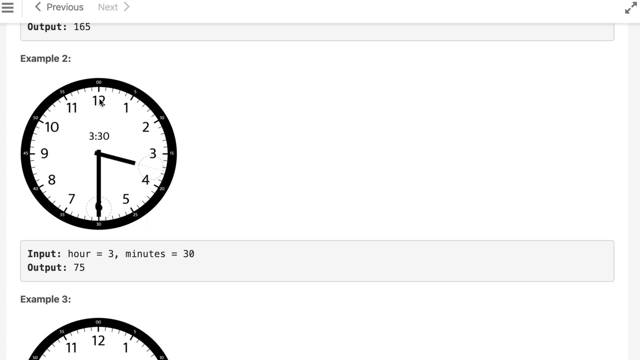 in in some decimal values, So we will keep it float. So total hour is this given hour, which is integer, And we will keep modular 12, since our is from one to 12.. But if it's 12, that is, if it's here, it's zero. 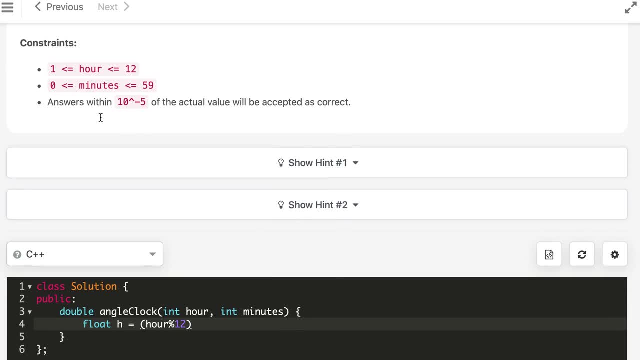 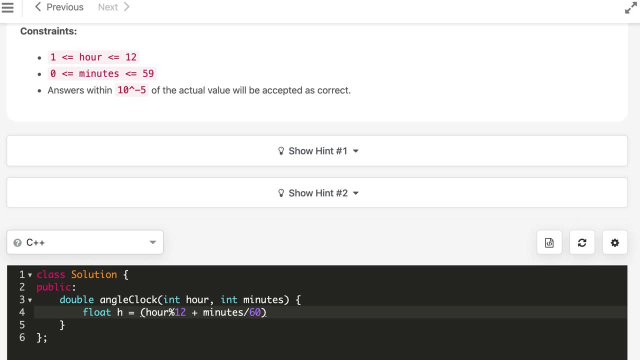 In fact we are keeping this as a reference, So we will keep 12 as zero. Others will remain same. So our modular 12 plus minutes divided by 60.. So this will be the fractional hour and this is integer. So if you divide by 60, this entire thing will be integer and it will always be. 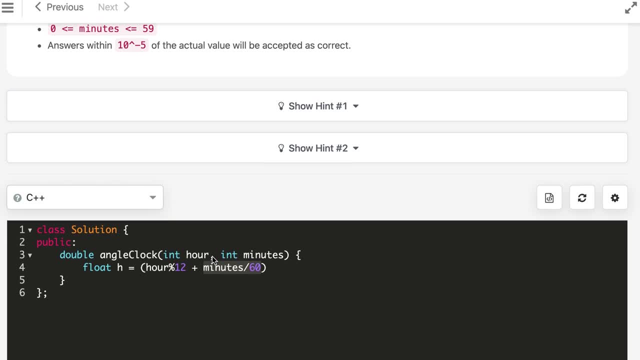 zero, since minute is maximum 59. So this will always be zero. So better to convert it to float and then this multiply by 30. So 30 comes from three 60 divided by 12, that is three 60 divided into 12 hours. 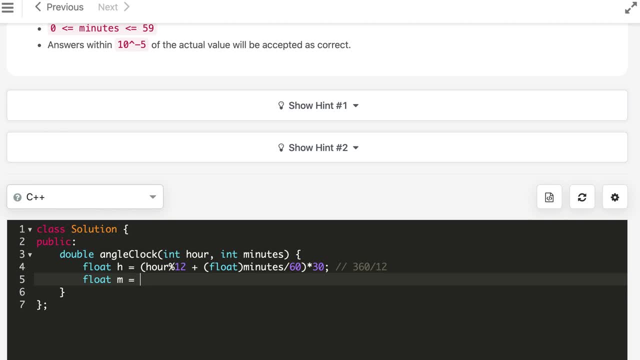 And then The Position of minute handle is minutes multiplied by six, And this comes from three, 60 divided by 60, three, 60 divided into 60 minutes And float angle equal to you will take the absolute values H minus M. 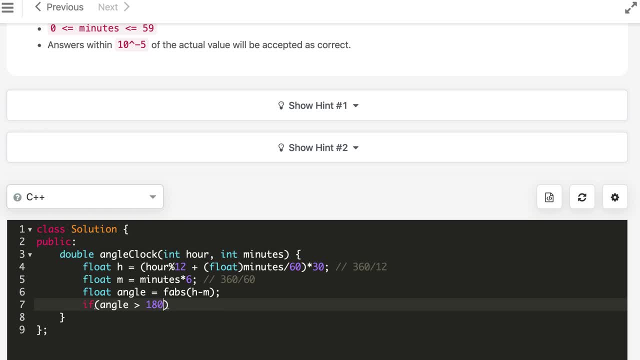 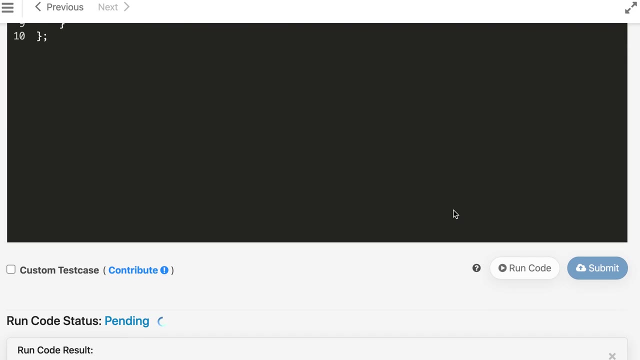 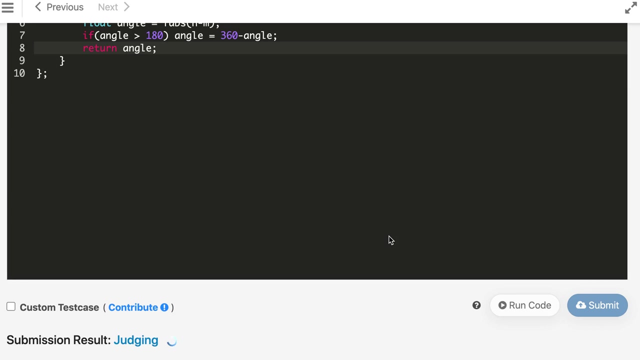 And if angle is more than one- 80, then angle equal to three, 60 minus angle, And finally we will return angle and let's see, And the answer matches. So let's submit And the solution is accepted And it's zero millisecond. 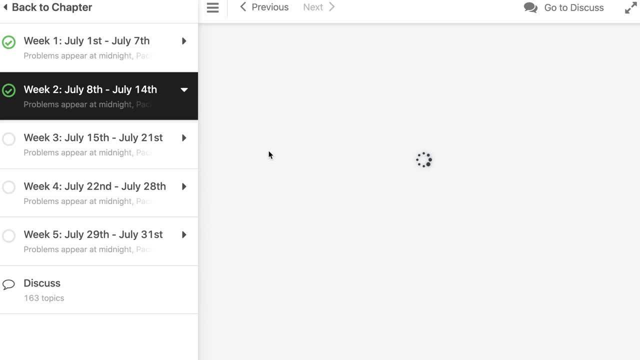 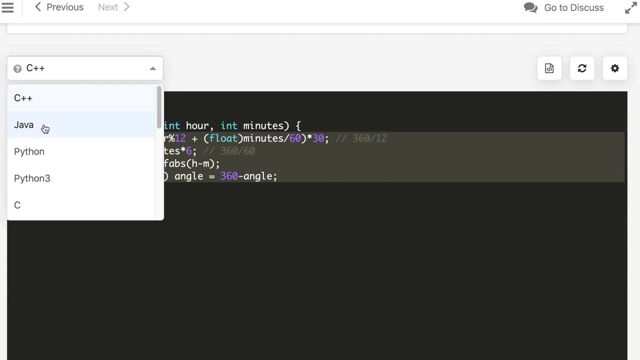 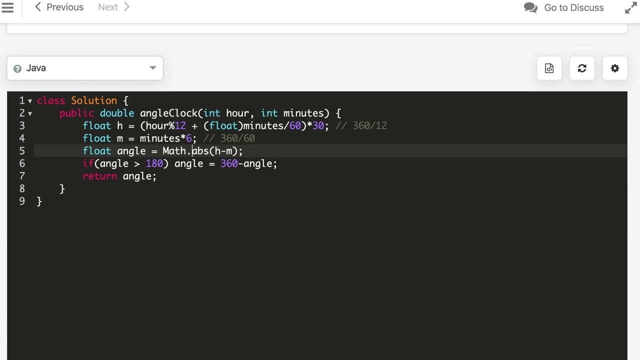 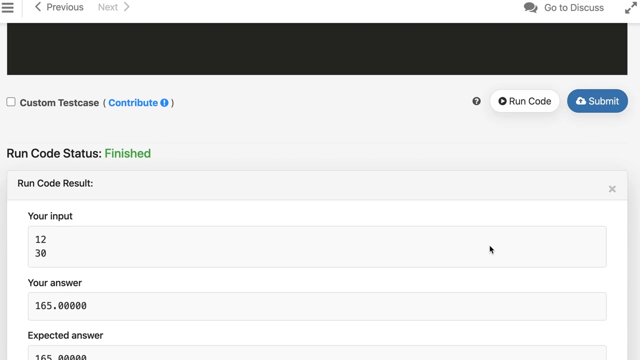 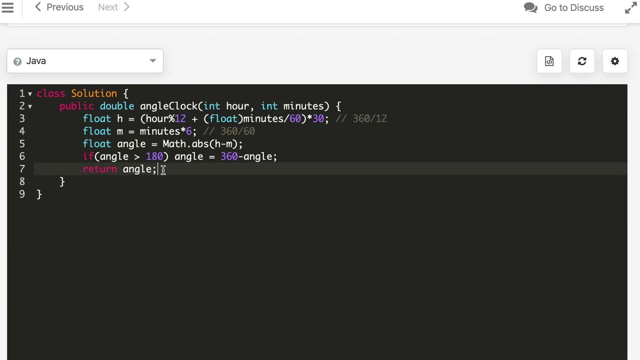 That is. uh, it's good, So it's constant time. not much trick here. We are just doing a few calculations and the same thing would be in Java, So let's do it Onto ask」. And the solution is accepted in Java as well.